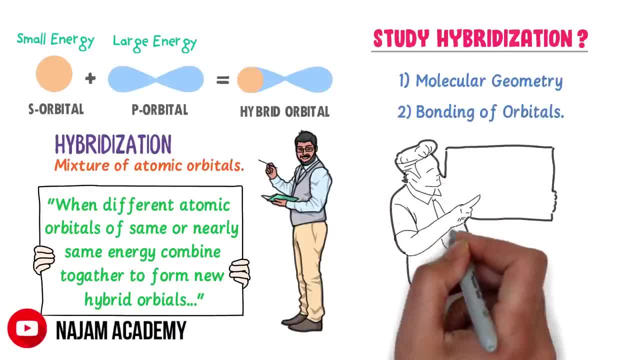 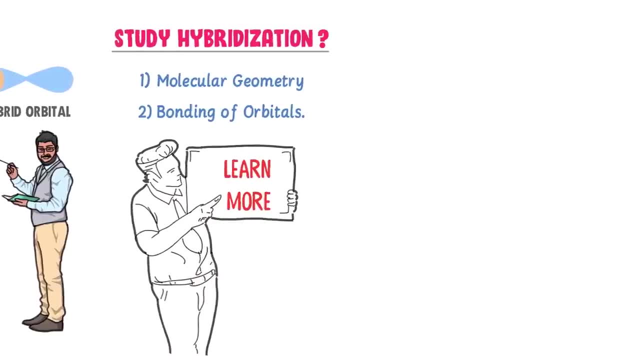 it shows us the bonding of atomic orbitals. You will learn more about the molecular geometry and bonding of atomic orbitals in this lecture. Secondly, why atomic orbitals are hybridized Are why hybridization of atomic orbitals is called hybridization of atomic orbitals. Well, you will. 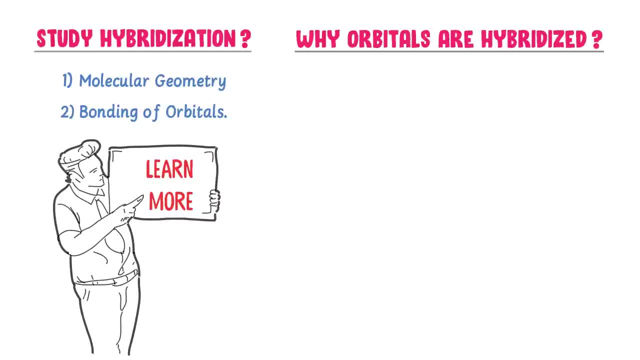 learn that. why hybridization of atomic orbitals is called hybridization of atomic orbitals? Well, there are different theories which explain this concept, but I am going to explain it very easily. Consider two types of atoms: A-atom and B-atom. Let A-atom has two orbitals. 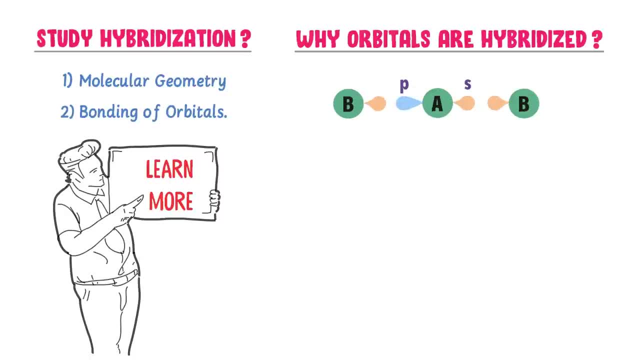 s-orbital and p-orbital, while B-atom have only one orbital, like s-orbital. Now let A-atom react with two atoms of B to form a molecule. We can see that there is s-s-bond between A-atom and B-atom, while here is s-p-bond between A-atom and B-atom. 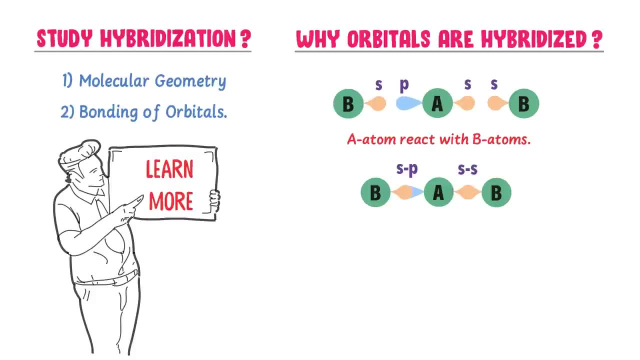 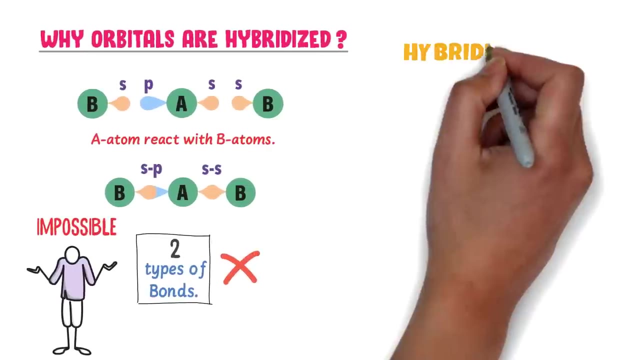 We can see that s-s-bond is totally different from s-p-bond. It means that A-atom forms two types of bonds with the same atom of B, which is impossible, not understandable and 100% wrong. Thus, to solve this issue, we look at the hybridization of atomic orbitals. 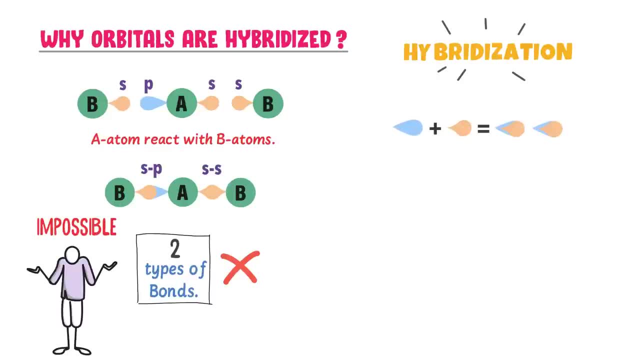 our mixture of atomic orbitals, Now s-orbital and p-orbital, would combine together to form two hybrid orbitals known as sp-orbitals. Here this is sp-orbital and this is also sp-orbital. Hence this sp-orbital of A-atom will form covalent bond with s-orbital of B-atom. 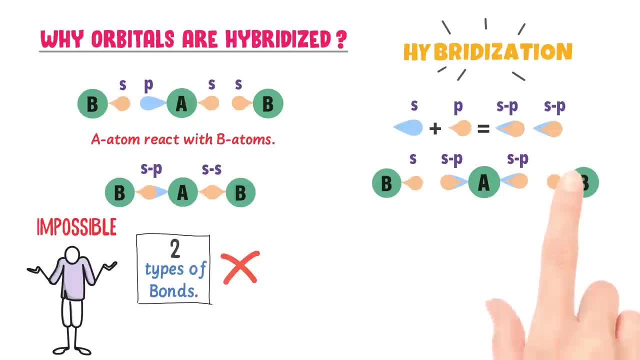 and this sp-orbital of A-atom will also form covalent bond with s-orbital of this B-atom. So this is now s-sp-bond and this is also s-sp-bond. Now we can say that A-atom forms s-sp-bond. 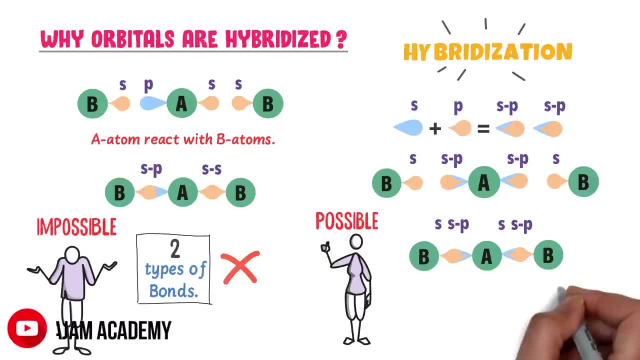 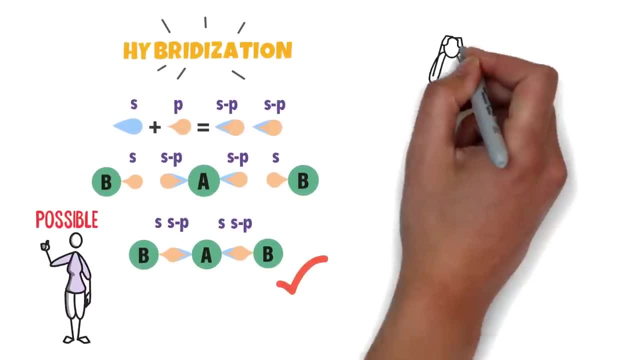 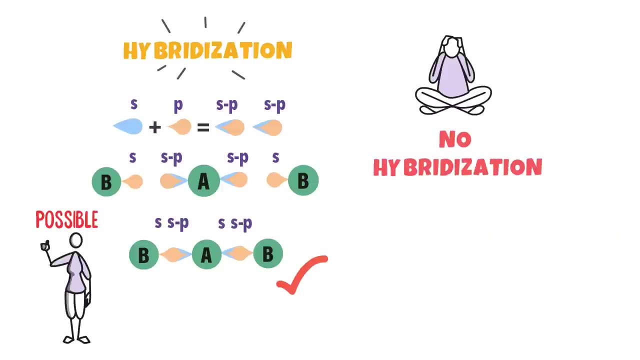 with B-atom, which is possible, understandable and 100% right. Also, remember that hybridization of atomic orbitals does not take place in every molecule. For example, no hybridization occurs in the atomic orbitals of molecules like H2,. 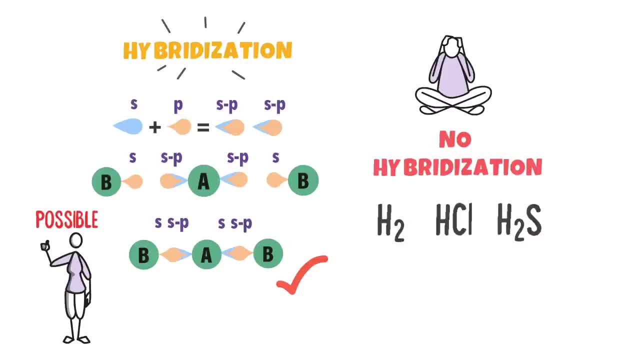 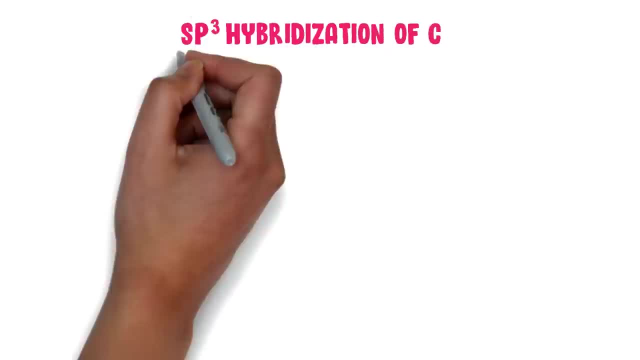 HCl, H2S, etc. Now let me explain the hybridization of atomic orbitals of carbon. Firstly, learning sp-3 hybridization of a carbon atom. Sp-3 hybridization means that in this mixture of atomic orbitals there is one s-orbital and three p-orbitals. 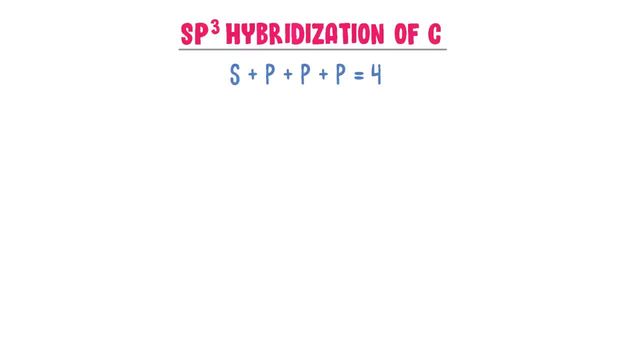 So there are total four orbitals present in sp-3 hybridization. There is 25% s-character and 75% p-character present in the sp-3 hybridization. Know how 1s and 3p orbitals combine together. 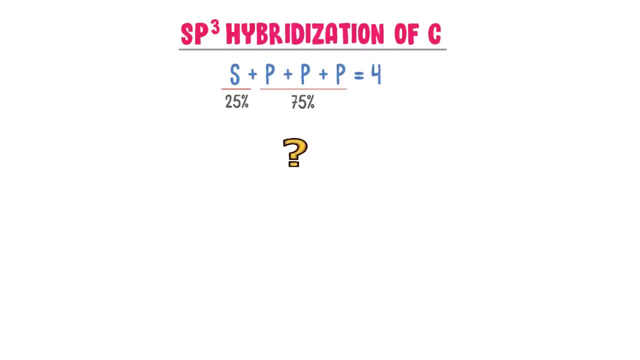 to form sp-3 hybridization. For example, consider a carbon atom in the ground state. We know that there are six electrons present in a carbon atom. In 1s there are two electrons and in 2s there are two electrons. 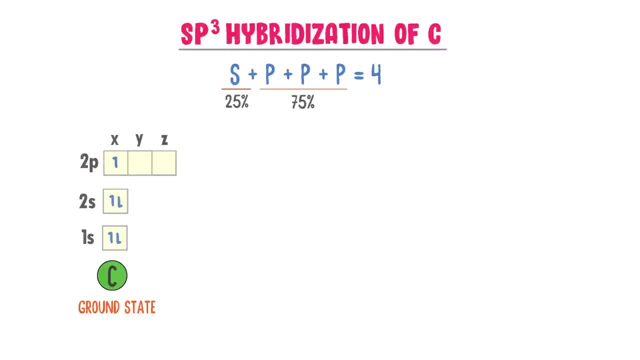 While In 2p there is one electron in the x orbital and one electron in the z orbital. Moreover, both 2p and 2p are läpse. Soक and 2p are لاpse, And an atom is either 1 or dB. So, assuming that we consume aтом of either transfusion ofuais of carbon study. 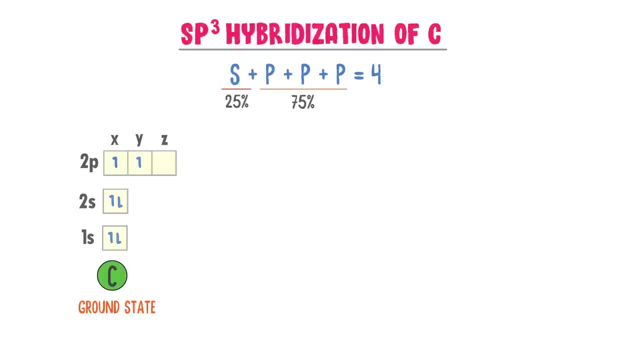 we know that there are 6 electrons present in carbona atoms and there are points ofostaje of carbon that form sp-3 hybridization orbital and one electron in the y orbital. Now let consider the excited state of a carbon atom. There are two electrons in the 1s orbital, While the one electron and two s jump into. 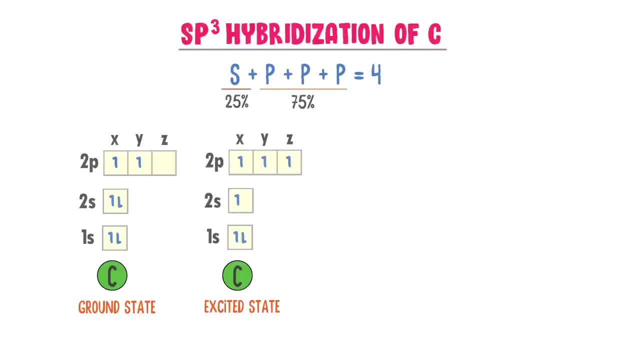 z orbital of 2p. this is the excited state of a carbon atom. The 1s orbital is already complete, having two electrons. So this 2s orbital and three orbitals of 2p, x, y, z mix are combined together to form four hybrid orbitals. Thus I will place these unpaired 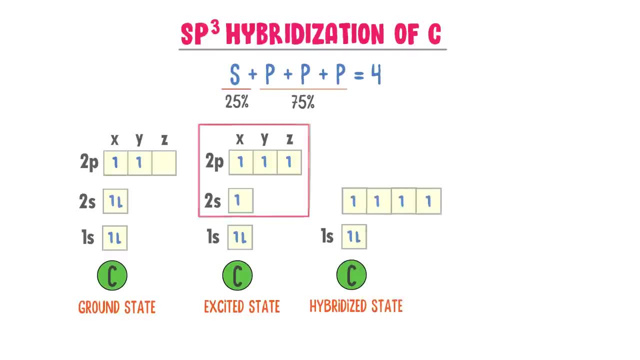 four electrons and these four hybrid orbitals. Remember that they must have the same spin. This is the first sp3 orbital, this is the second sp3 orbital, this is the third sp3 orbital and this is the fourth sp3 orbital. So we have four hybrid orbitals, sp3 each. 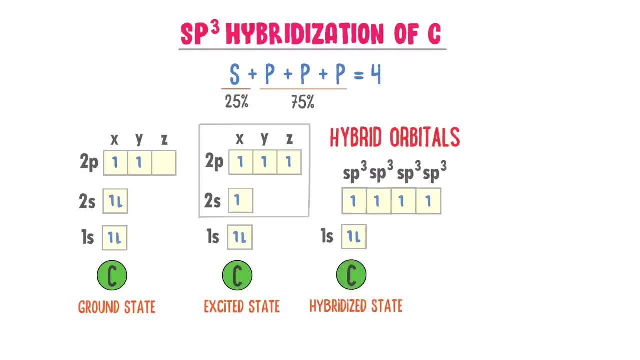 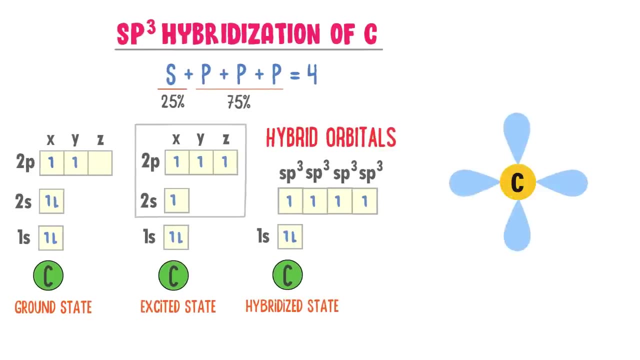 having one electron. Now it is sp3 hybridization That teaches us the geometry of carbon and its molecule. For example, carbon has this type of geometry and sp3 hybridization. This is one sp3 orbital. this is second. third, 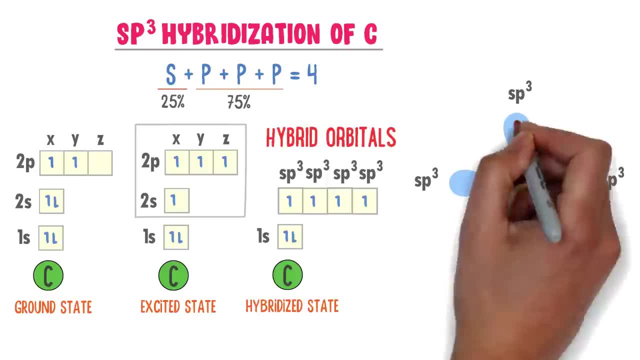 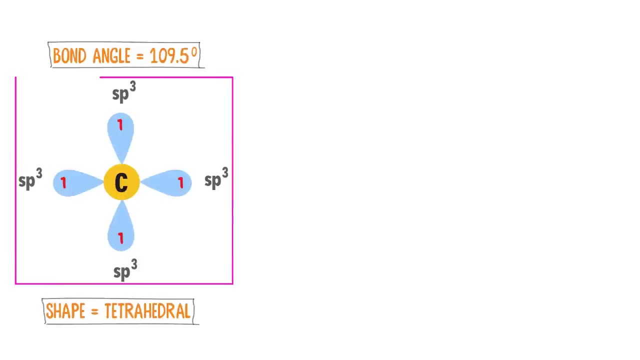 and fourth sp3 orbitals and each orbital having single electron. The bond angle in sp3 hybridization is 109.5 degree and the ship of sp3 hybridization of carbon is tetrahedral. Note it down that these four sp3 hybrid orbitals are called degenerate orbitals. It means that 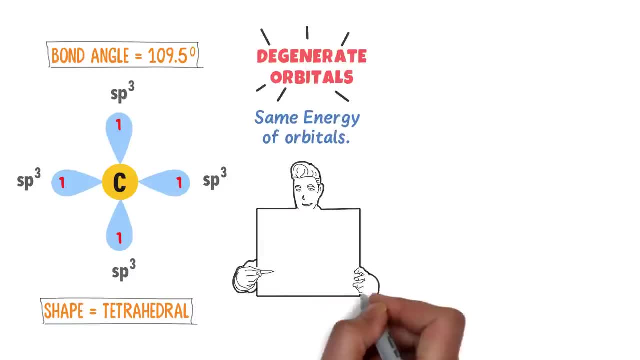 they all have the same energy. Also, let me give you an example of sp3 hybridization of a carbon and a molecule like methane CH4.. Now consider sp3 hybridization in this carbon atom. We know that there are four unpaired 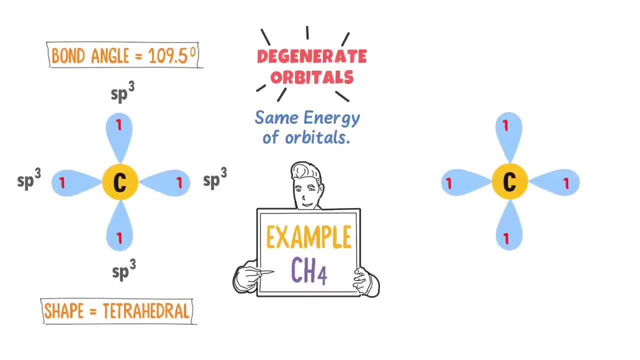 electrons present in it. According to valence bond theory, or VBT, the unpaired electrons are needed to form covalent bond. So four hydrogen atoms will share their single valence electron with the electron of hybrid orbitals of a carbon and we get 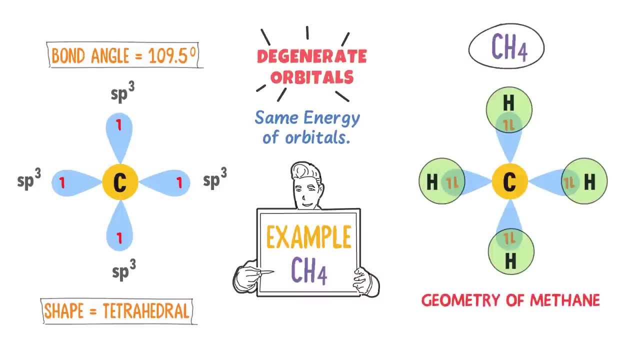 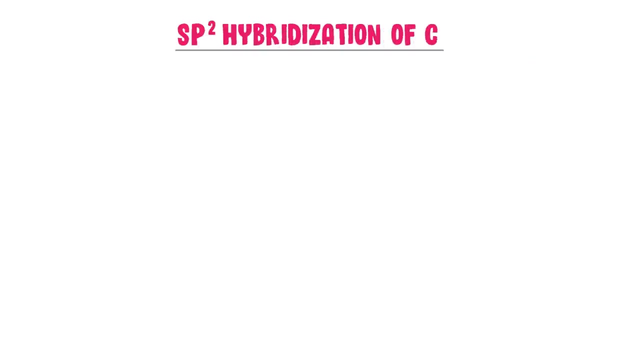 CH4.. Thus, this is the ship and geometry of methane CH4, in which carbon has sp3 hybridization. So note it down, this example. Secondly, let me teach you sp2 hybridization. Sp2 hybridization means that In this mixture of atomic orbitals there is one s-orbital and two p-orbitals. Hence, 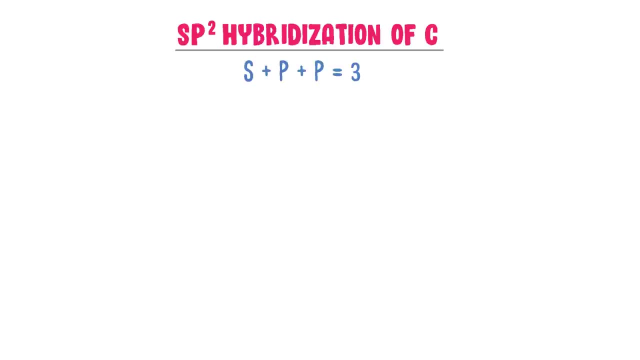 there are total three orbitals present in sp2 hybridization, or there is 33% s-character and 67% p-character present in sp2 hybridization. Now how these orbitals 1s and 2s combine together in sp2 hybridization. Well, again consider. 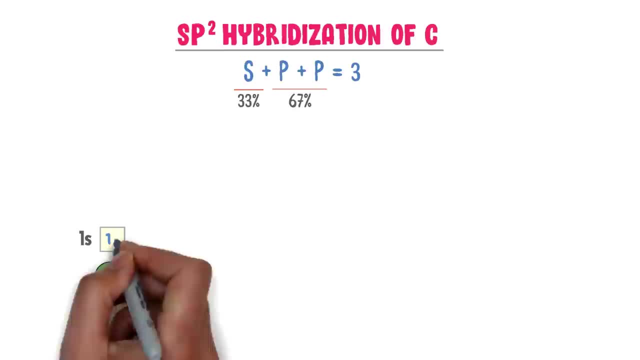 carbon in a ground state. We know that Now, for example, In a state 1s has two electrons, 2s has two electrons and in 2p there is one electron in x-orbital and one electron in y-orbital. 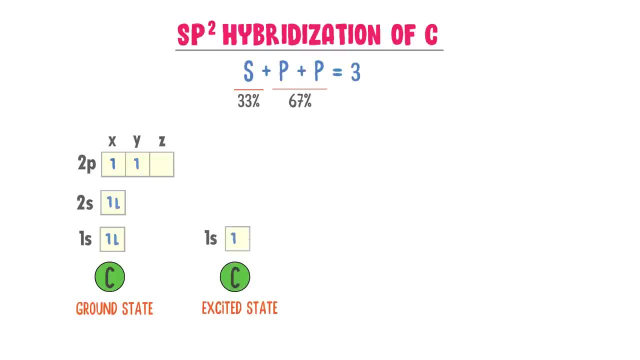 While in an excited state of carbon, 1s has two electrons, 2s has one electron and in 2p there is one electron in x-orbital, one electron in y-orbital and one electron in z-orbital. 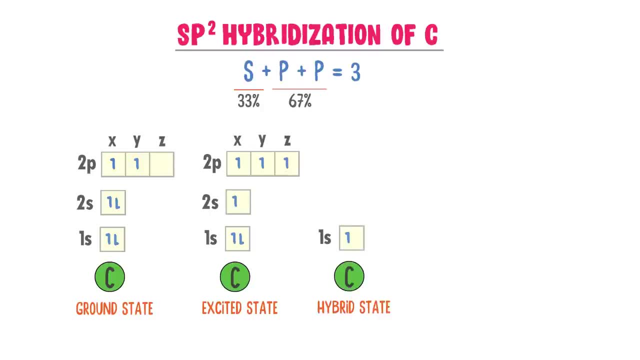 Now, in this hybrid state of offense, there are already two electrons present in 1s-orbital. Now I will promote the mountains heterogeneous, seperti these, aha and other blocks. We know that in sp2 hybridization one s orbital and two p orbitals combine together. 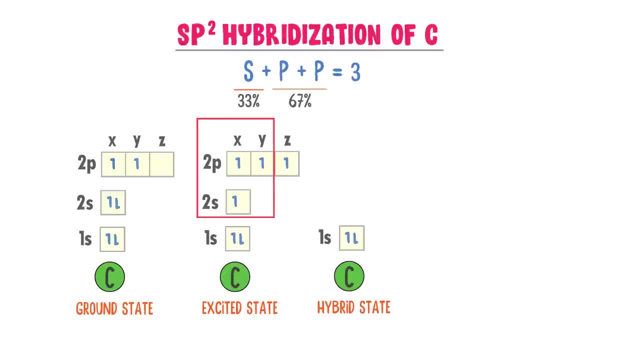 So this two s orbital, x and y orbitals of two p would combine together to form three orbitals of sp2 hybridization. Thus I will put these unpaired electron in these hybrid orbitals having same spin. This is the first sp2 orbital, this is the second sp2 orbital and this is the third sp2. 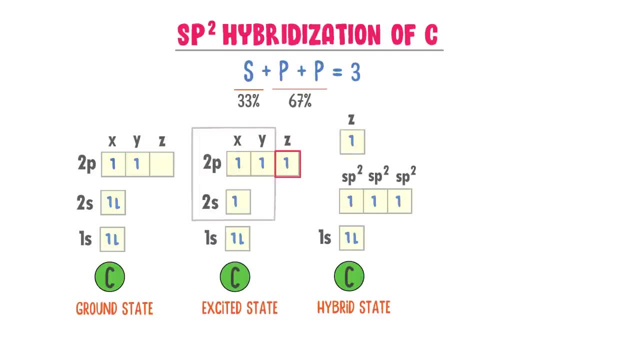 orbital. Lastly, I write this z orbital of two p here. This z orbital is unhybrid orbital. It means that this z orbital do not combine with two s, two px and two py. Also, it has more energy than all these three hybrid orbitals. 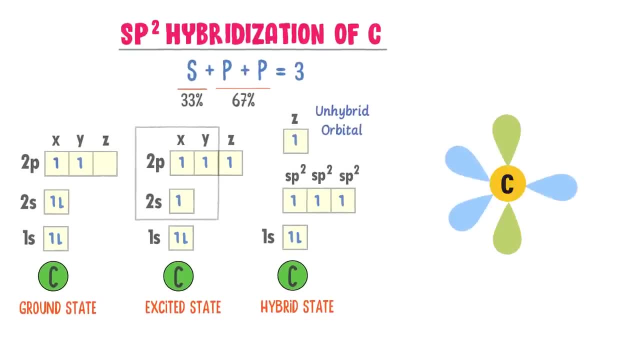 Now carbon has this type of geometry and sp2 hybridization. This is the first sp2 orbital. This is the second and third sp2 orbital, While this long orbital is the two pz orbital, which is unhybridized orbital. These all orbitals have one electron each. 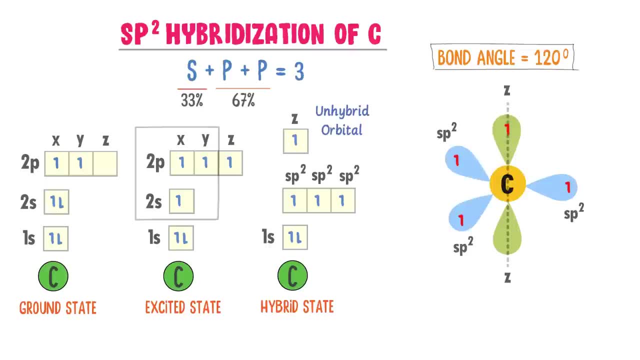 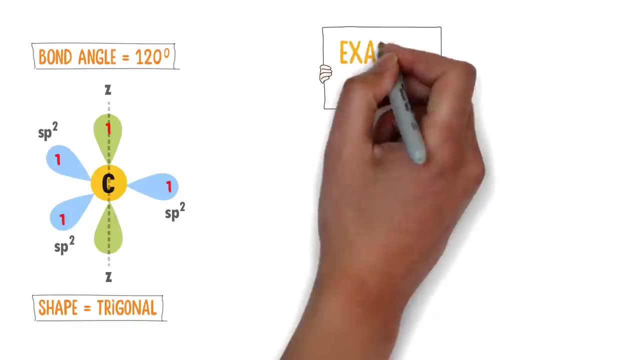 Remember that the bond angle in sp2 hybridization is 120 degree, while the ship of carbon is trigonal. Also, let me give you an example of sp2 hybridization of carbon in a molecule like ethane. Let consider sp2 hybridization and this carbon atom. 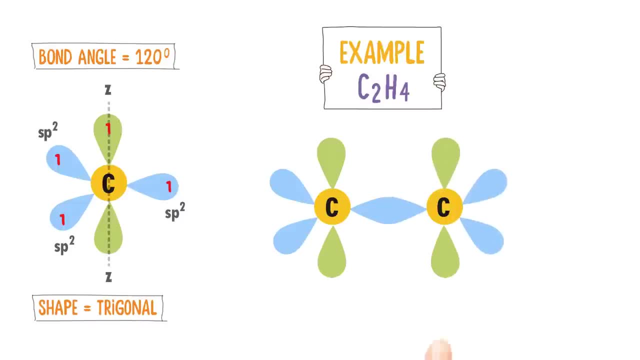 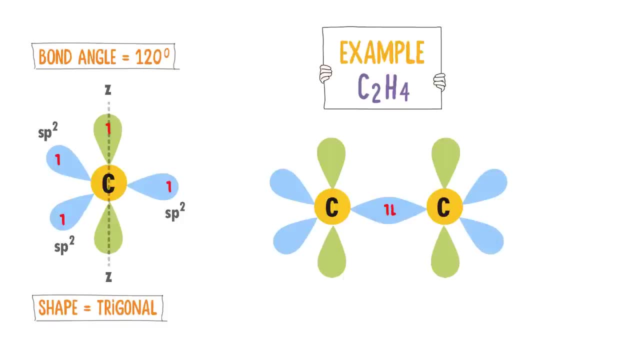 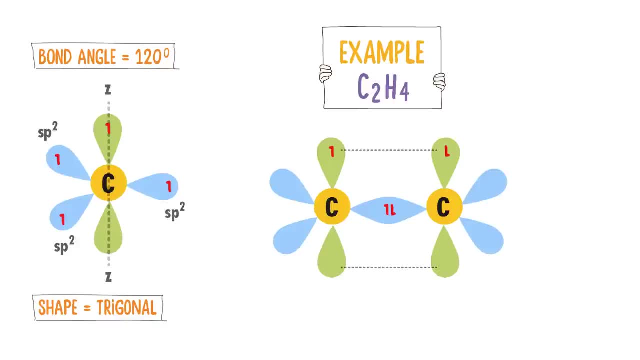 in the unhybrid orbitals to Pz. Then hydrogen will share its one electron with this sp2 orbital and with this sp2 orbital. Also, hydrogen will share its electron with this sp2 orbital and with this sp2 orbital. Note it down that unhybrid orbitals always form pi bond, For 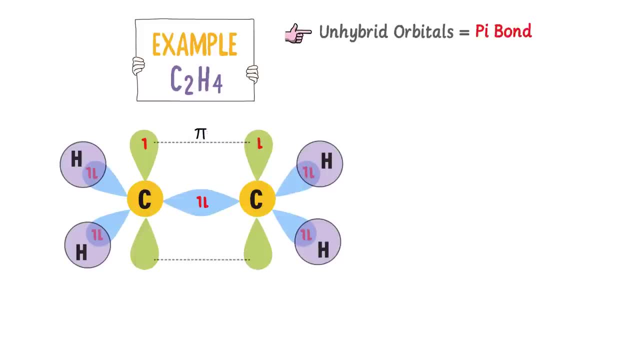 example, these two Pz form pi bond, while hybrid orbitals always form sigma bond. For example, these sp2 orbitals form sigma bond. Thus, in ethane there is one pi bond and one sigma bond between carbon-carbon atoms. Hence this is the shape and geometry of a molecule in 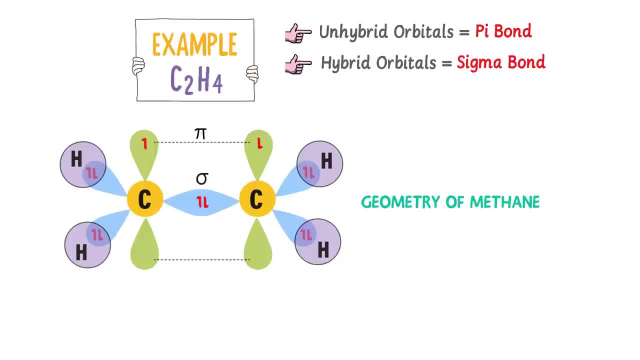 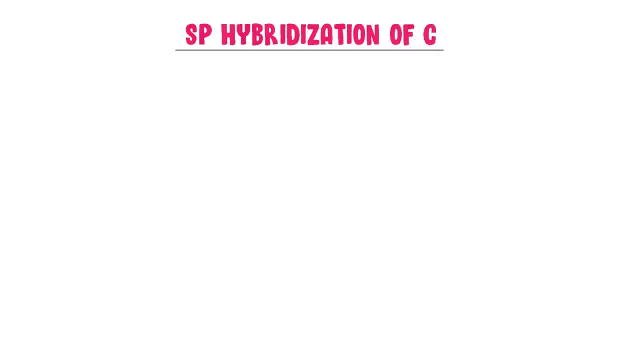 which carbon has sp2 hybridization. So note it down this example. Finally, let me teach you sp hybridization. Sp hybridization means that in this mixture of atomic orbitals there is one orbital of s and one orbital of p present in it, So there are total two orbitals present in sp. 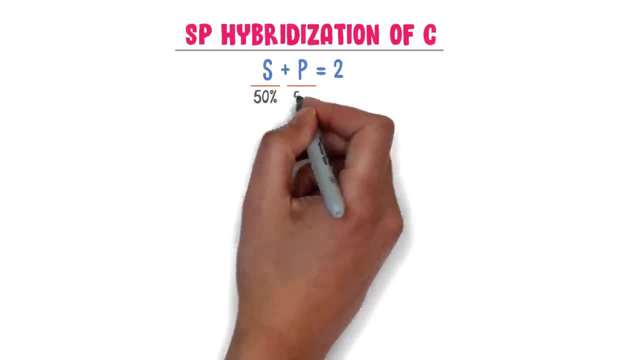 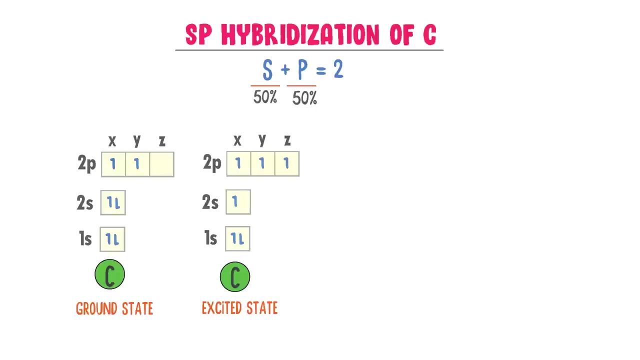 hybridization. There is 50% s-corrector and 50% p-corrector in it. Now how one s-orbital and one p-orbital combine together to form sp hybridization. Well, again, the contribution has to be shown by both these three elements per unit. 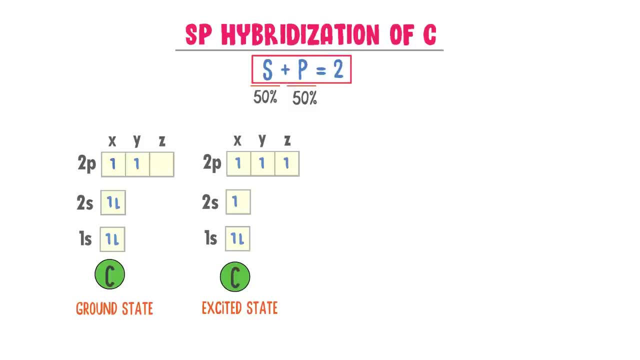 One that is also 100% p and one that is 5% p To obtain a results match. consider that a form is seen in the first sl service table, given by an orbital and vector in pr�-carboxyloy3-ggn as a method of convolution of a spin-shape. 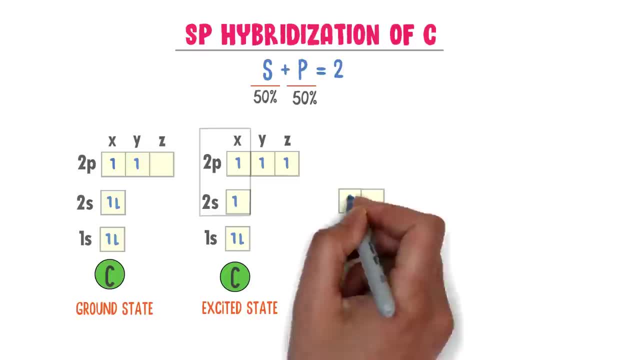 in a set of topics For now. you will learn that when we solve a problem or requirements which can refer to the punya class by treating a single set number of sub conductors, as also known as pickers. orbitals of 2p do not take part in sp hybridization of carbon, So they both are unhybrid orbitals. 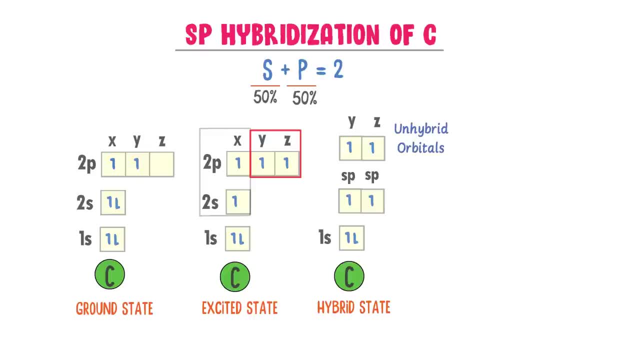 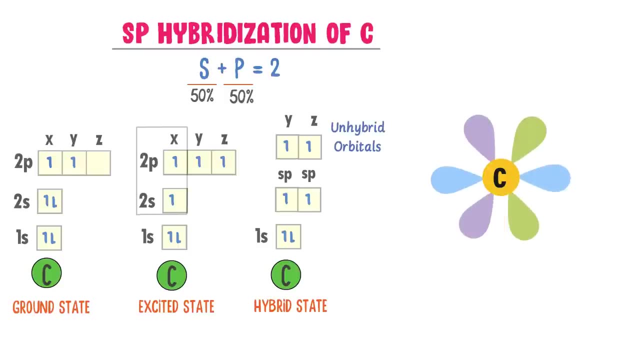 Thus we have two hybrid orbitals and sp hybridization, each having unpaired electron. Now carbon has this type of geometry and sp hybridization. This is the first sp orbital and this is the second sp orbital. While this long orbital is 2py and this long orbital is 2pz, They